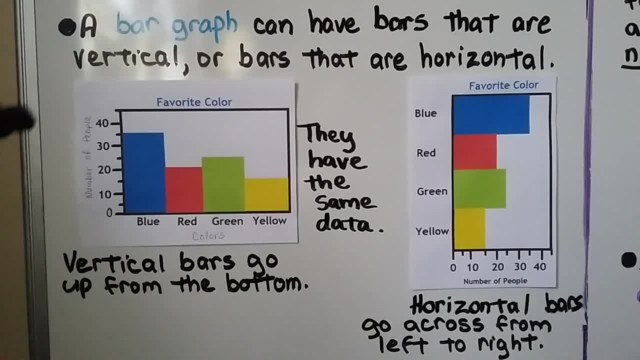 or bars that are horizontal. These bars are vertical. They go from the bottom up. See, They have the same data. These bars are horizontal bars and they go across from left to right. They start on the left and they go towards the right as the numbers get bigger. If we look here, we can see. 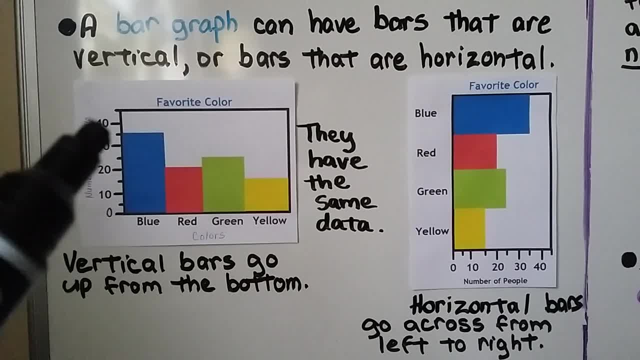 here's 40 and it's in the middle, so it must be 35. And on this one, blue is at 35.. Red is at 20.. This red one is at 20.. This green one is in between 20 and 30, so it must be 25.. This green one is also 25.. 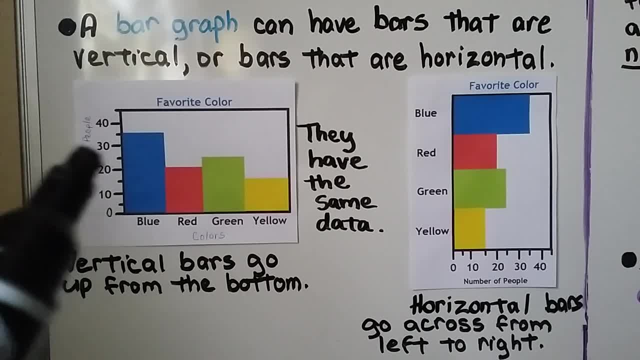 This yellow one is in between the 10 and the 20, so it must be 15.. And this yellow one is 15.. They have the same data. One has vertical bars that go up from the bottom and this one has horizontal bars that go across from left to right And just like a frequency table or a tally table. 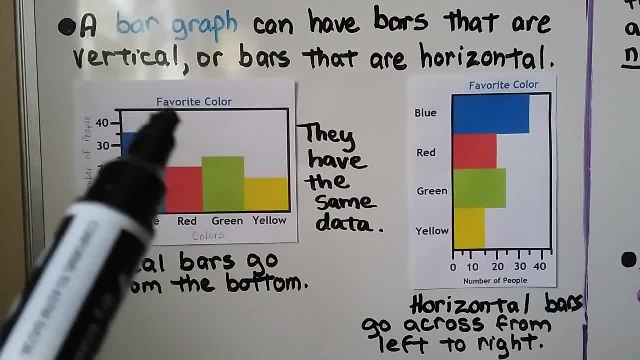 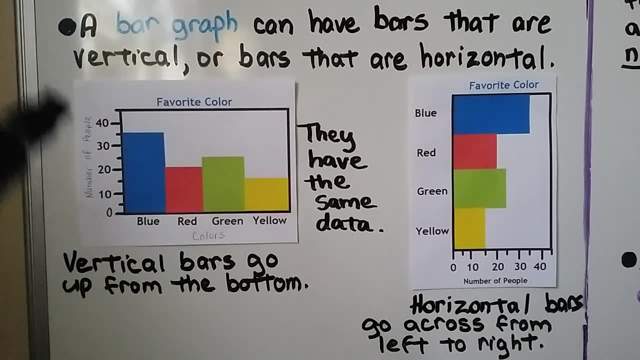 or a picture graph. we can see it has a title up here and the words are: each word is capitalized. We can see it's labeled for the scale of what the scale is counting and we can see it's labeled at bottom for what the answers are. This bar graph shows favorite pets and here's the. 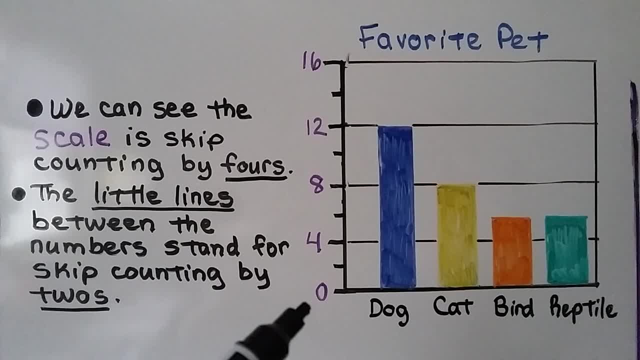 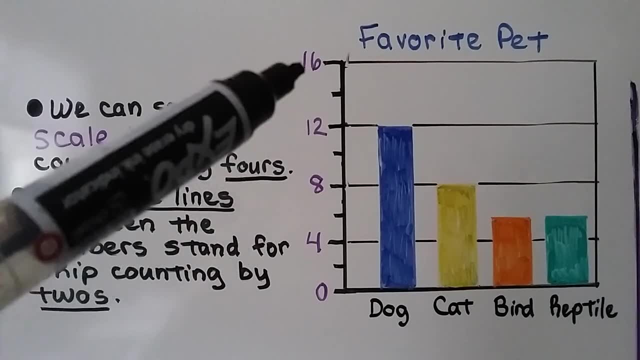 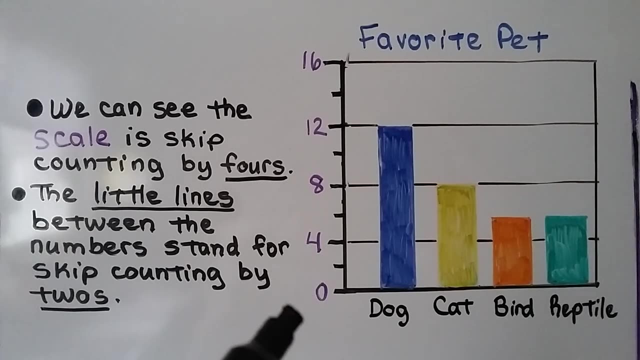 answers that the people gave. We can see this scale is skip counting by fours. It goes from 0,, 4,, 8,, 12, to 16.. The little lines in between the numbers stand for skip counting by twos. If that's a four and this is in the middle, it's halfway. 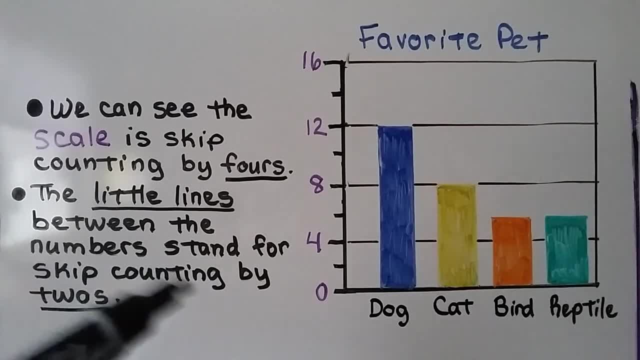 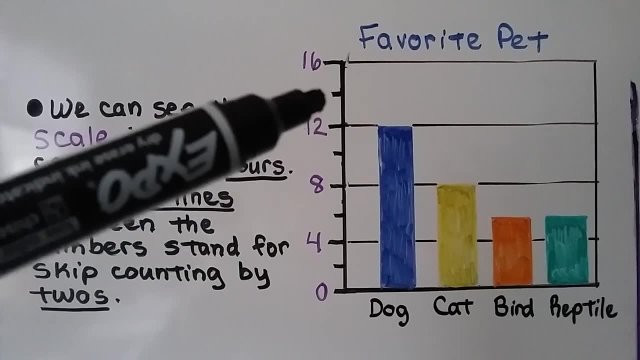 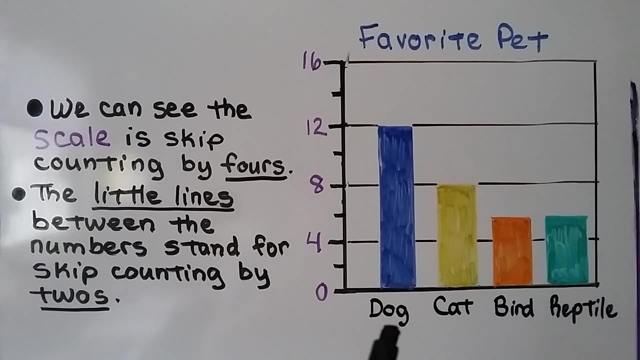 it must be half of four, so it's a two. We could say 0,, 2,, 4,, 6,, 8,, 10,, 12,, 14,, 16, skip counting by twos, We can see 12 people chose dog as their favorite pet. Eight. 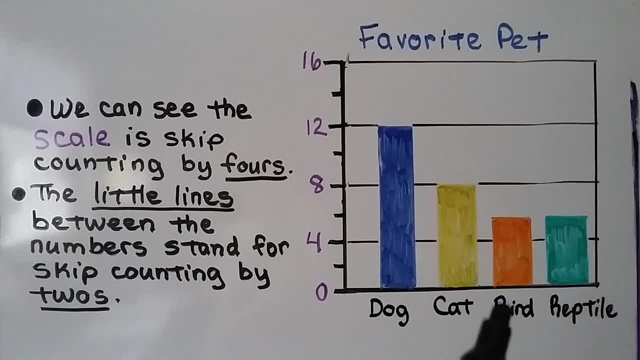 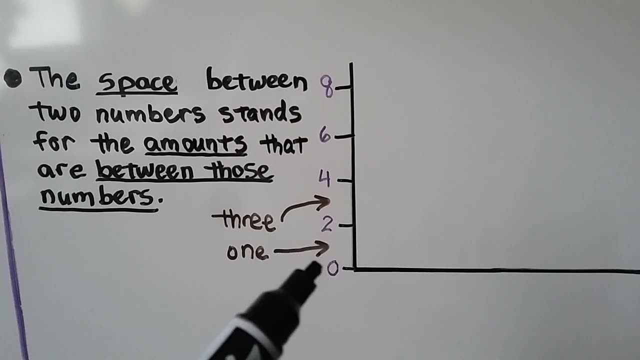 people chose. cat and bird is in between four and eight, so it must be six, and reptile is also six. Sometimes there won't be little lines in between the scale numbers, It'll just be an open space. The space between two numbers stands for the amounts that are between. 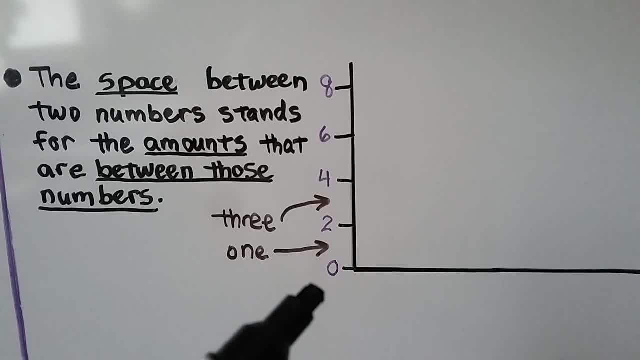 those numbers. This scale is: skip counting by twos, Zero, two, four, six, eight. So we know. if a bar was right here in the middle, that means the answer is a 1.. And if the bar is right in the middle here, it must be a 3.. 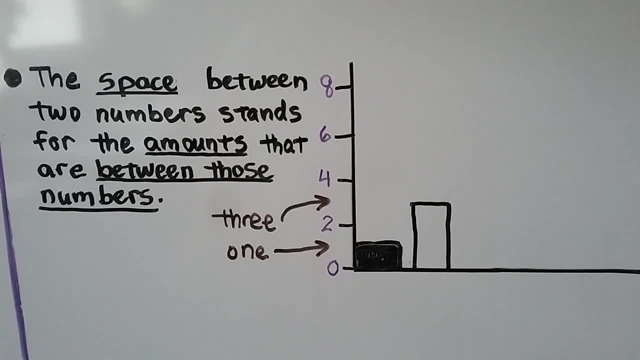 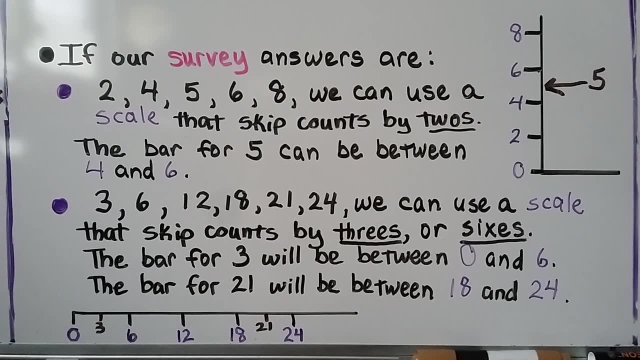 We would know the answer was 3.. It's in between the 2 and the 4.. If our survey answers are a 2,, 4,, 5,, 6,, 8, we can use a scale that skip counts by twos. 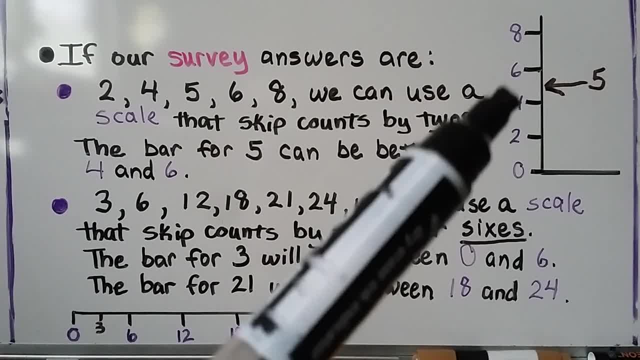 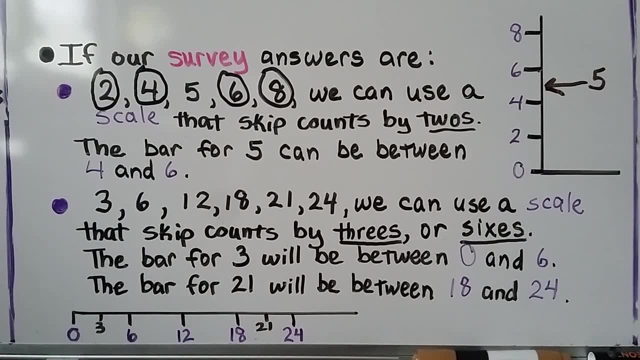 We would have 5,, the bar for 5, in between the 4 and the 6.. But all the other numbers are numbers that skip count by twos. The only one that doesn't skip count by twos is the 5.. 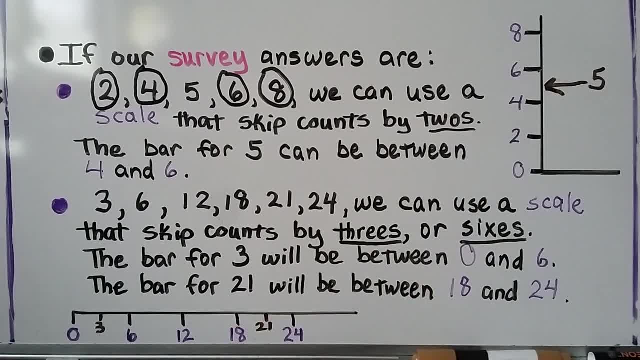 And we can use a bar that goes in between for that one, But all the others skip count by twos. so that would make sense: 3, 6,, 5.. 12,, 18,, 21,, 24.. 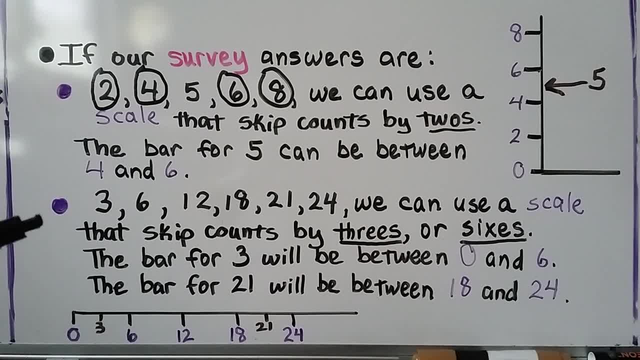 We can use a scale that skip counts by threes or sixes. If we skip count by sixes, the bar for 3 would be in between 0 and 6. And the bar for 21 would be in between 18 and 24.. 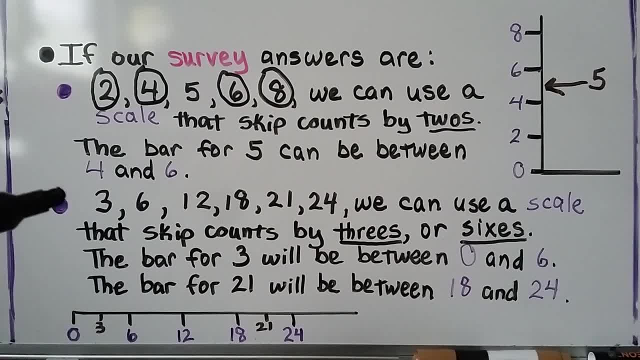 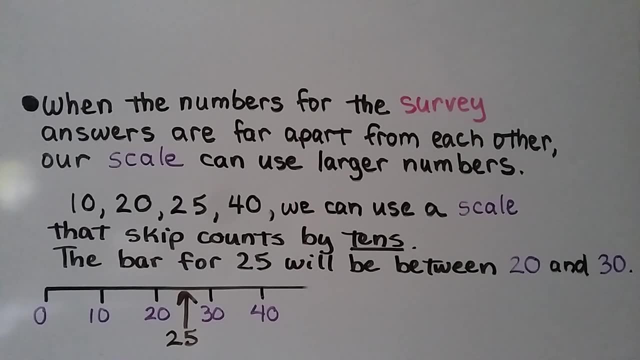 So for these numbers we could use a scale that has skip counts, Skip counting by threes or sixes. either one would work. When the numbers for the survey answers are far apart from each other, our scale can use larger numbers If we have numbers like 10,, 20,, 25,, 40,. 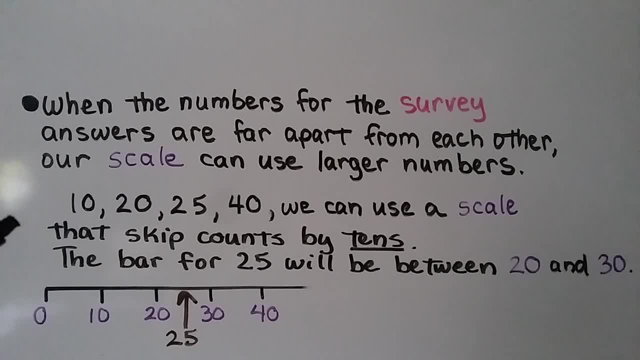 we can use a scale that skip counts by tens: 10, 20,, 30,, 40.. 10, 20,, 30, 40. The bar for 25 would be in between the 20 and the 30.. 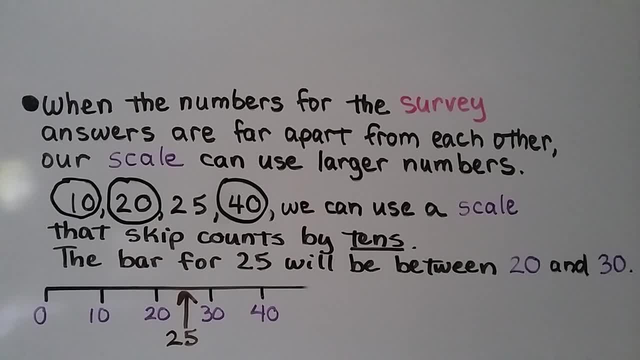 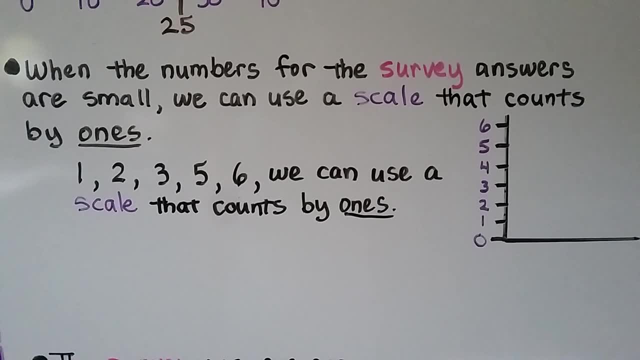 Some survey answers can be very large, like in the hundreds or thousands. even When the numbers for the survey answers are small, we can use a scale that counts by ones If our answers are 1,, 2,, 3,, 5, and 6,. 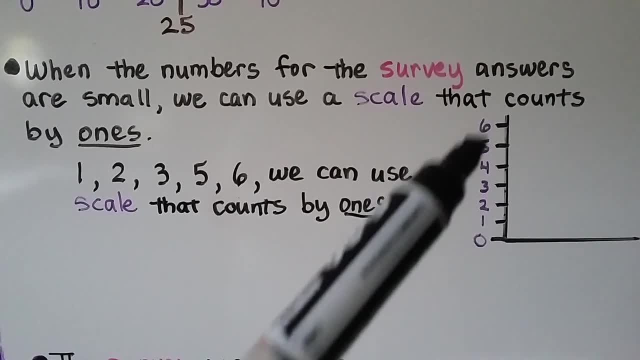 we can use a scale that counts by ones. Starts at 0.. 1,, 2,, 3,, 5, and 6.. Starts at 0.. 1,, 2,, 3,, 4,, 5,, 6.. 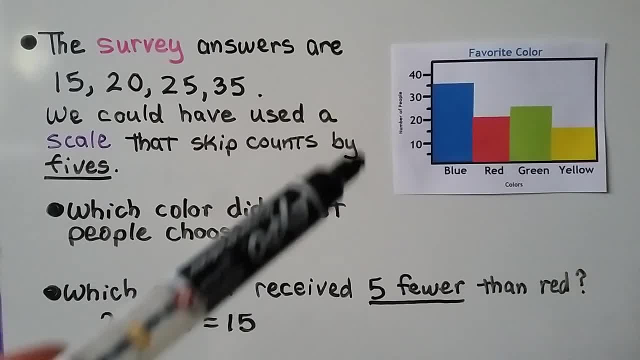 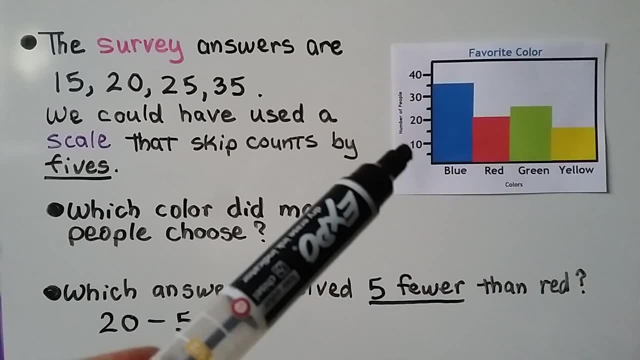 This bar graph is about favorite colors. This is the number of people that answered. Here are the colors, the answers that people gave. We can see it skip counts by 10.. 10, 20,, 30, 40.. Because the answers are 15, 20,, 25,, 35,. Because the answers are 15,, 20,, 25,, 35,. because the answers are 15,, 20,, 30,, 40,. Because the answers are 15,, 20,, 25,, 35,, we couldn't get 2.. 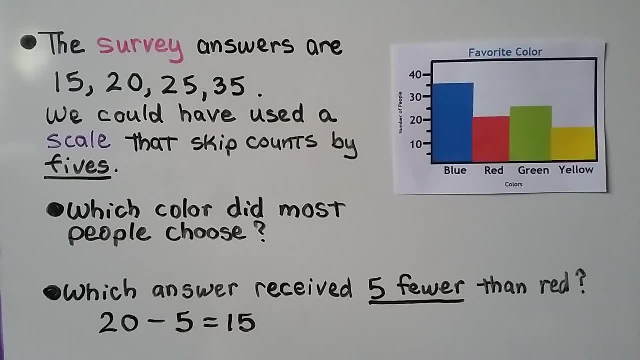 we could have used a scale that skip counts by fives. Bar graphs make it easy to see data. Just by looking at this bar graph can you tell which was the most favorite color? Which color did people choose the most? We can see that this bar is the tallest. 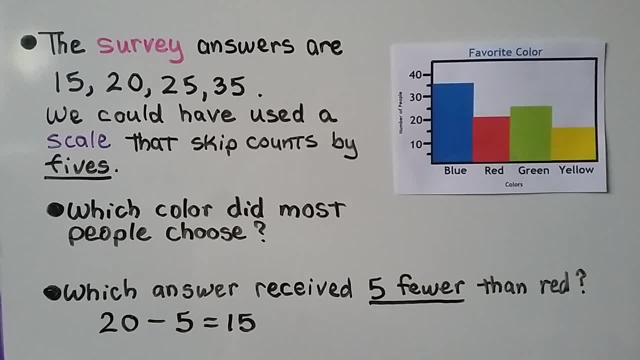 so that one has the most answers. blue. Can you see which one is least? We look for the shortest one. it would be yellow. Which answer received five fewer than red? We look for red. it's a 20.. If we're looking for five fewer. 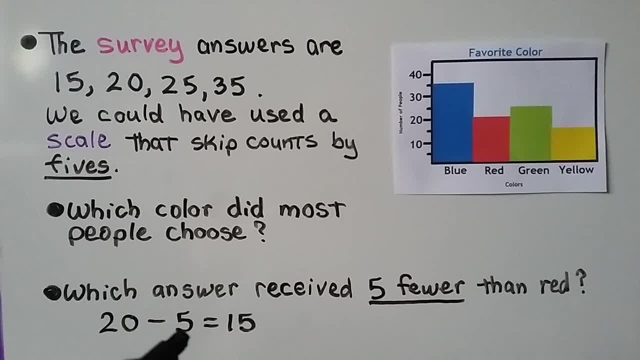 that's a clue to subtraction: 20 minus five fewer is equal to 15.. So which one had 15 as the number of favorite colors? We look on our scale. here's 15, that matches yellow. The answer is yellow. 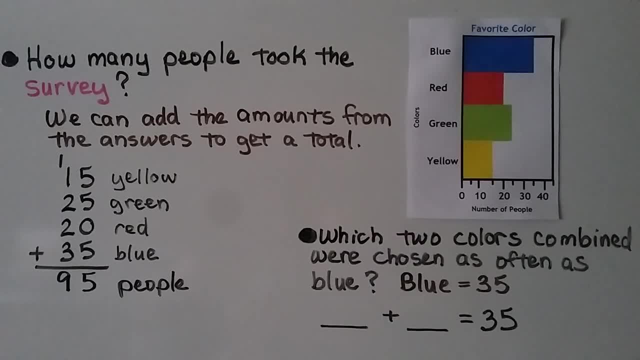 So here we have our bar graph of favorite colors. How many people took the survey? We can add the amounts from the answers to get a total. Yellow is 15.. Green is 25.. Red is 20.. And blue is 35.. 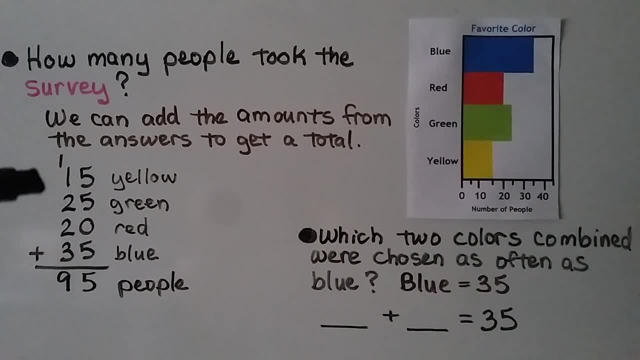 We add all the numbers of answers: 15 plus 25 plus 20 plus 35. Starting in the ones place we have: five plus five is 10, plus five more is 15.. We regroup the 10 from the 15,. 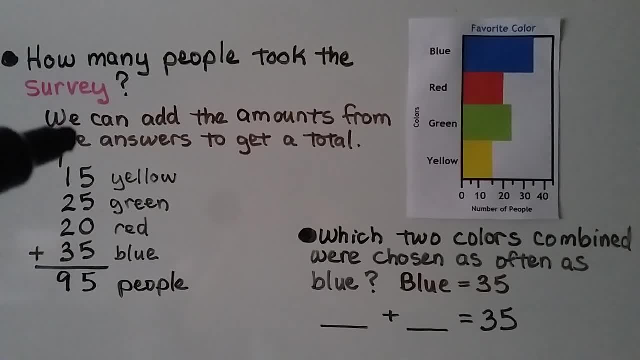 cause, that's a 10 and five ones, isn't it? We regroup the 10 to the tens place and put our five ones down. Then we add the tens column. We have three, four, five, six, seven, eight, nine. 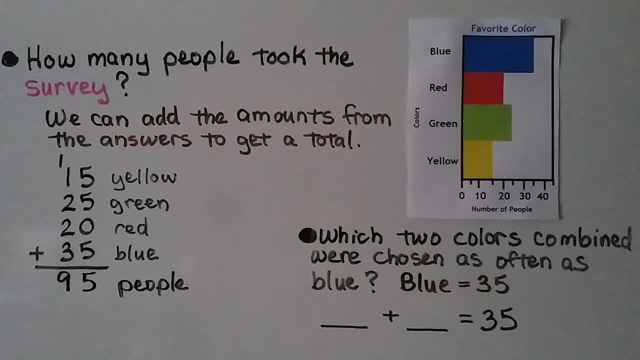 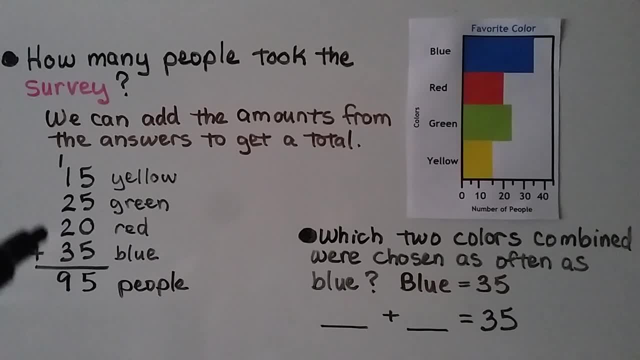 two that will equal 35.. Can you see two of these that will equal 35?? We can use the scale, we can use the math we just did. Which two colors have answers that would equal 35?? If you said red 20 and yellow 15,. 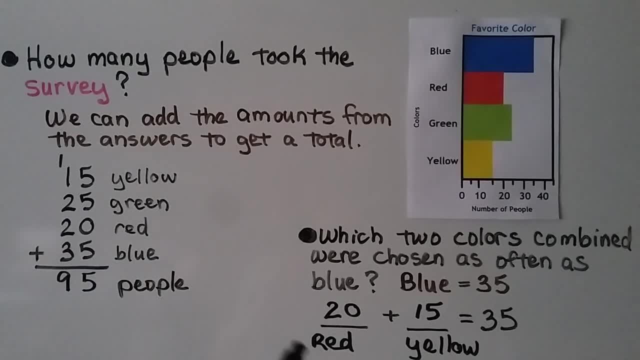 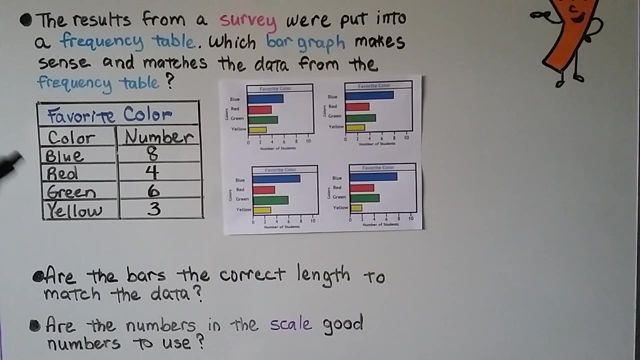 you're right. The red answers plus the yellow answers would equal 35.. 20 plus 15 is equal to 35.. The results from a survey were put into a frequency table. Remember, frequency tables use numbers. Which bar graph, which one of these bar graphs makes sense? 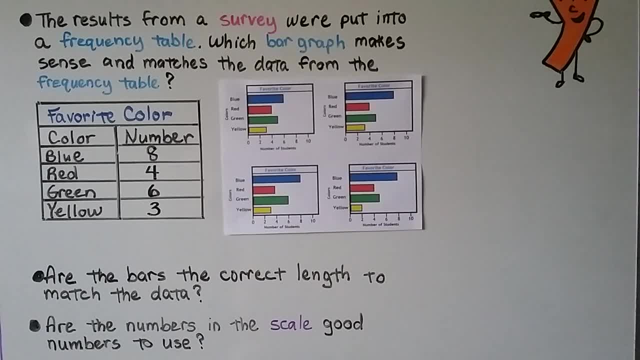 and matches the data from the frequency table. So we're going to look closer at these. but we need to see: are the bars the correct length to match the data? Are the numbers in the scale good numbers to use? So let's take a closer look. 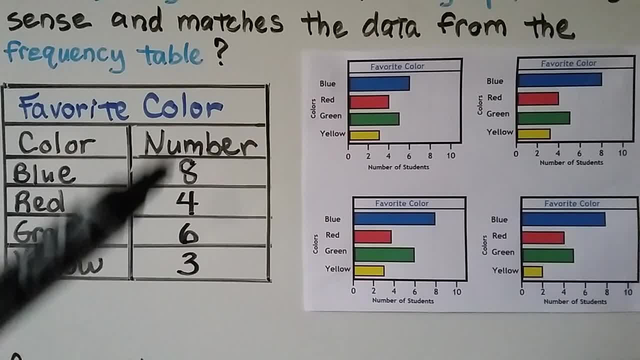 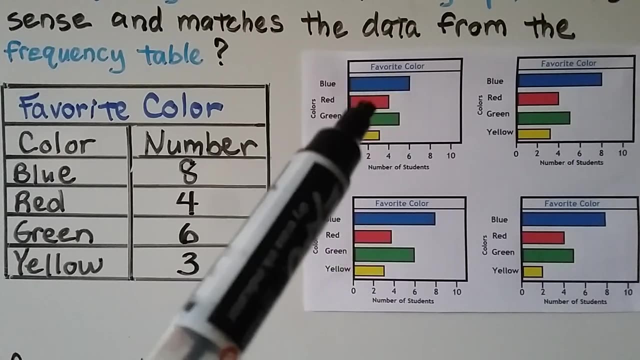 They're all about the same thing: Favorite color. they all have the same answers: blue, red, green or yellow. but it needs to match this frequency table. The first thing I see is blue should be eight. This one says blue is six, so it's not this one. 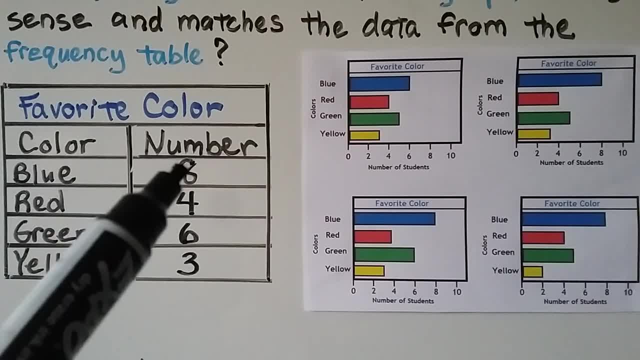 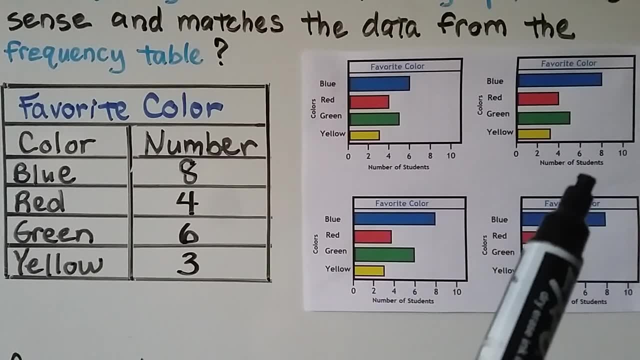 All the numbers have to match, And if blue doesn't match, well, then that's not all the numbers. So let's try this one. Blue needs to be an eight. Yes, this one has blue as an eight. Red needs to be a four. 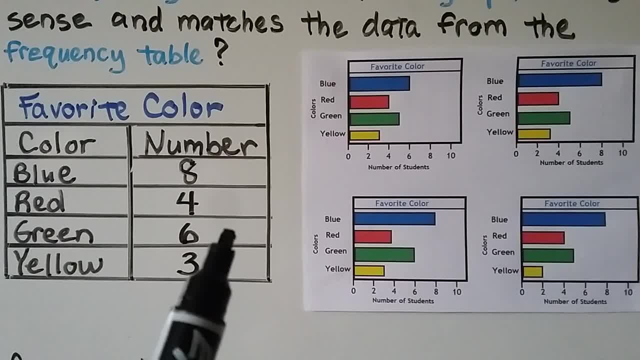 Yes, red is a four. Green needs to be six. Hmm, this green is in between the four and the six. That means it must be a five. So that's not the right one, because the green bar is wrong. What about this one? 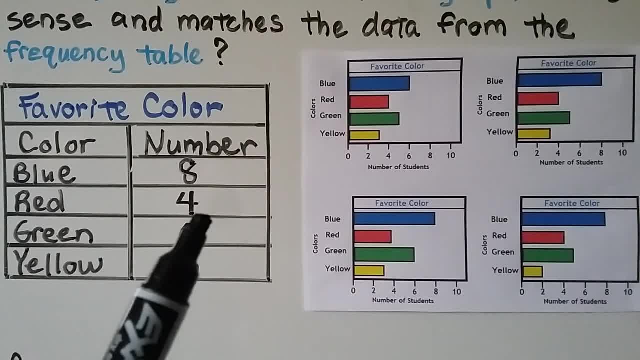 Blue needs to be eight- Yes, it's eight. Red needs to be four- Yes, it's four. Green needs to be six- Hmm, it's a five again. And yellow is supposed to be three, and it's only a two. 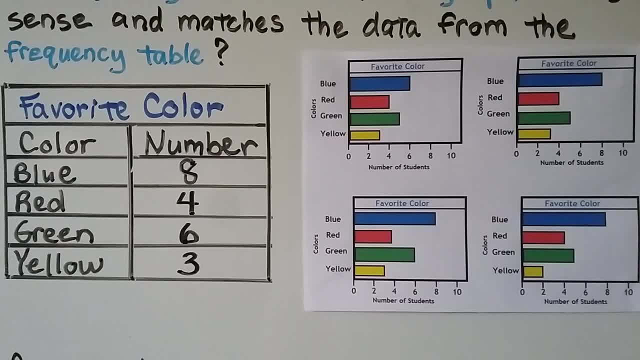 So that one's not right. This is the only one left. It must be the correct one. but let's double check to be sure. Blue is an eight, red is a four, green is a six and yellow is a three. 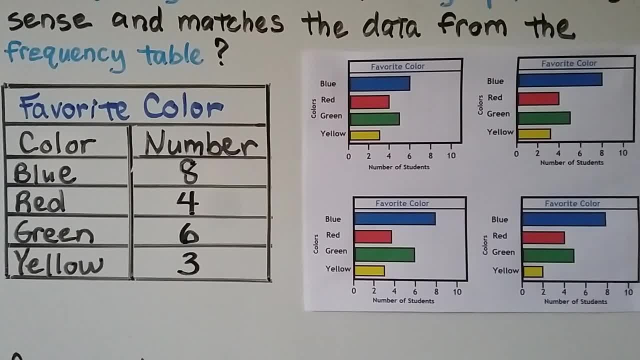 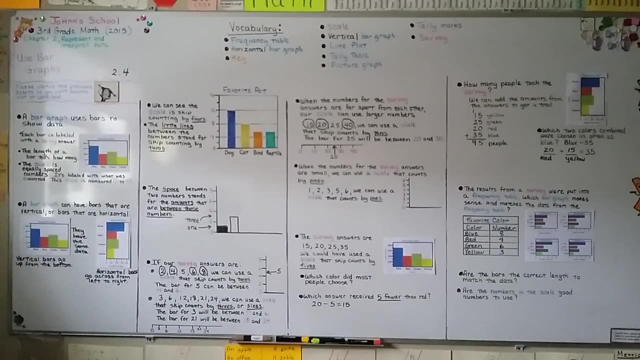 So this is the correct bar graph that matches that frequency table. They all have to match. All the answers have to match the numbers from the frequency table. In our next lesson we're going to make some bar graphs. You can make a survey and ask your friends and family.